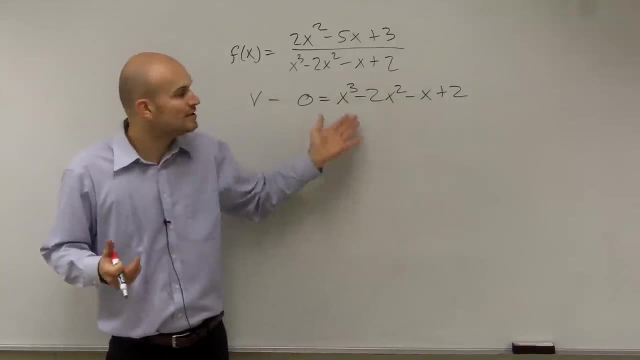 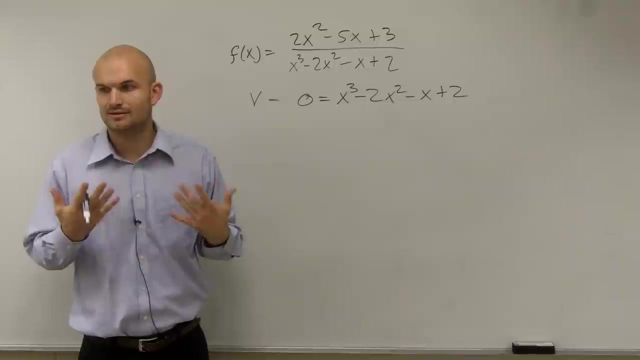 techniques. It's not a linear equation, so you just can't solve for x. You have multiple x's and when you have four terms, a factoring technique we use when we're doing a problem and you have four terms is factoring by grouping. So what you're going to want to do is group. 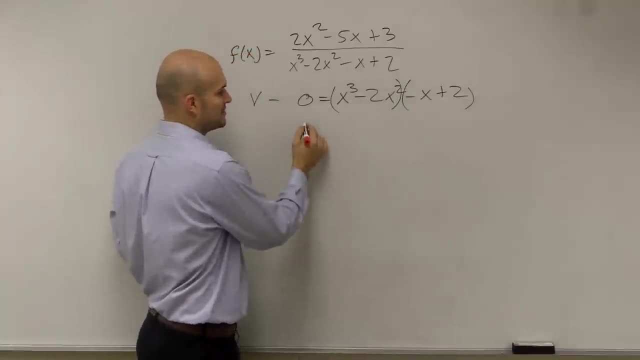 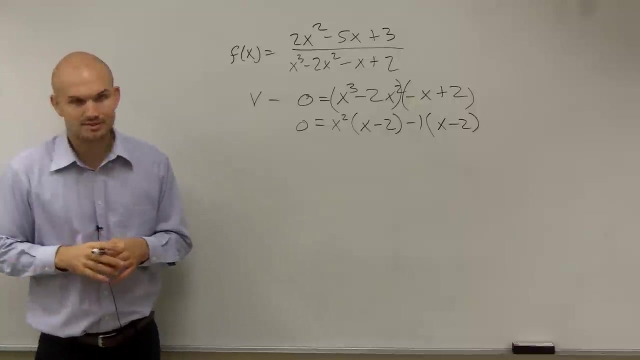 the first two terms and group the last two terms, Then factor out separately. So zero equals x squared times x minus 2.. Here I can factor out a negative 1, so therefore x minus 2.. Does everybody follow me with the grouping? Remember this from old school. Then we have. 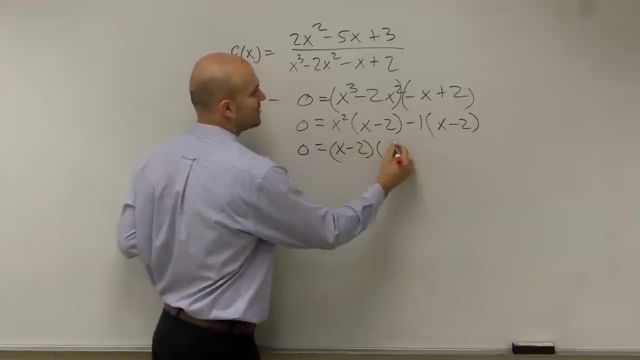 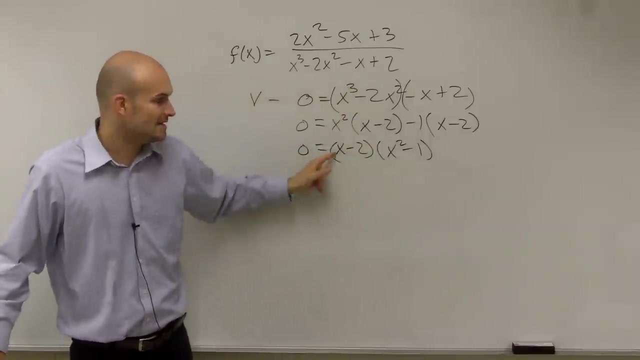 zero equals x squared minus 2.. X minus 2, I factor that out, so I have x squared minus 1.. Now the reason why we use factor: by grouping 1, I can group those two. factor it out. Now I can use the zero product. 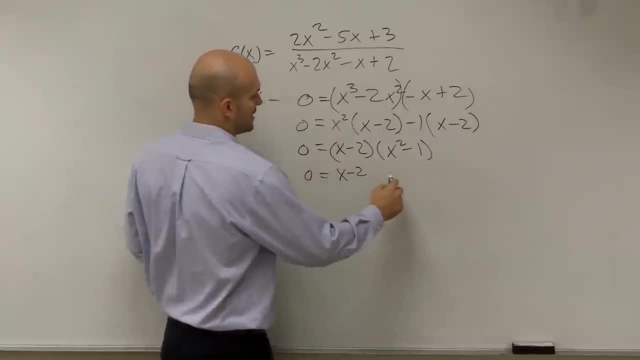 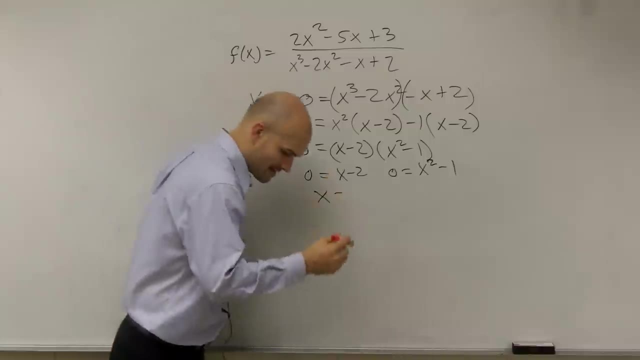 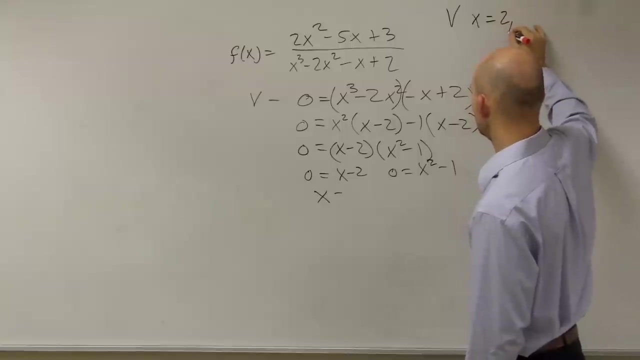 property and I can say: zero equals x minus 2, and zero equals x squared minus 1.. So my vertical asymptotes- which I'm actually going to write up here because I'm going to have to erase this- My vertical asymptotes are: when x equals positive 2, and 1 equals x squared, 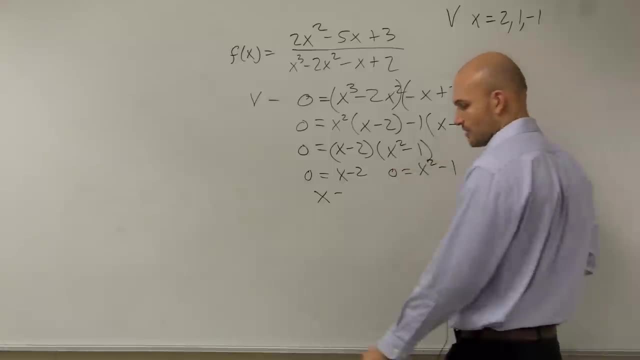 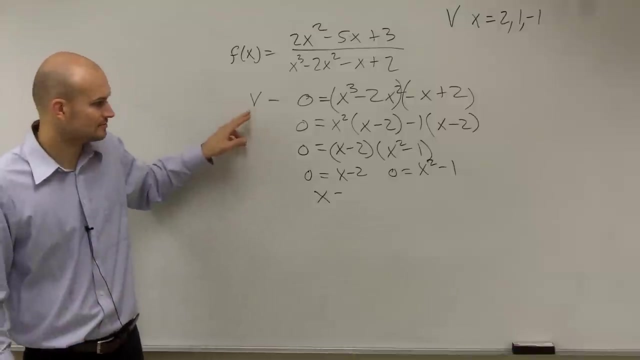 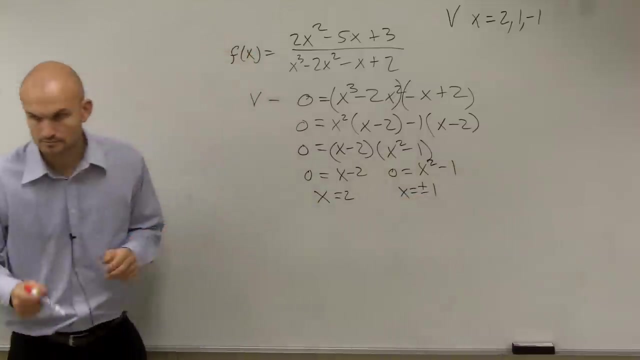 minus 1, and negative 1.. As I solve, I add 1 to the other side, take the square root and I get plus and minus 1.. Any questions with that? That was your vertical asymptotes. So x equals 2,, x equals plus or minus 1.. Cool with that. That's your hardest factoring problem. 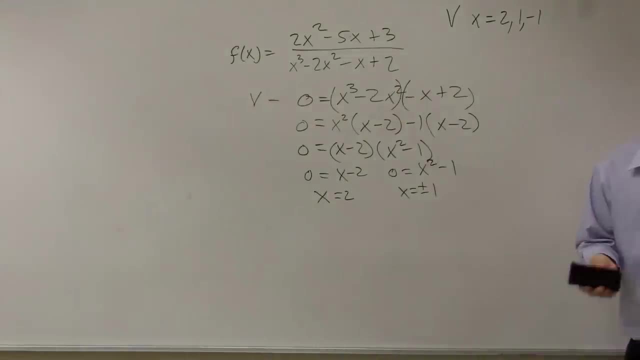 The rest of them out of your homework are: either you can solve just by solving an equation or you can solve by factoring a trinomial and so forth. So the next thing I need to do is determine. I'll do horizontal here next, while some of 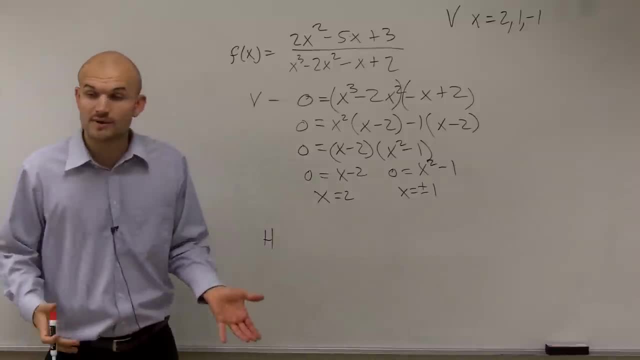 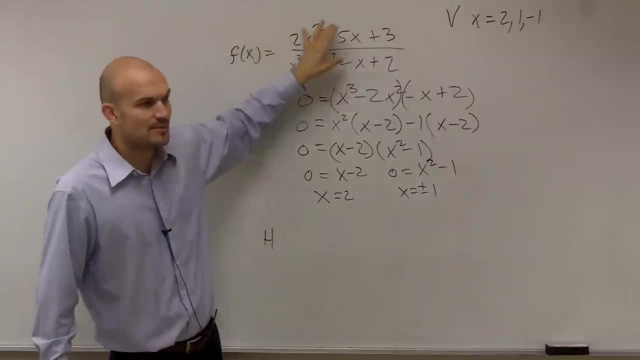 you are writing this down. So the next thing is horizontal. So the horizontal. I have to use my horizontal zero test. Remember, the horizontal zero test tells you to compare your exponents. So I make sure that my polynomials are in descending order with the highest. 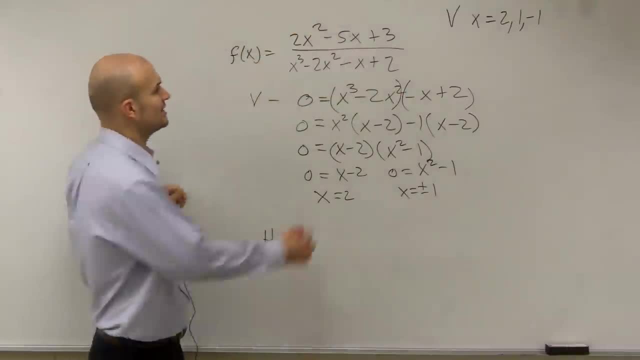 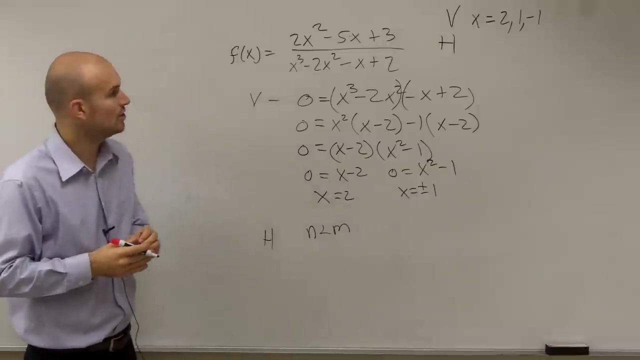 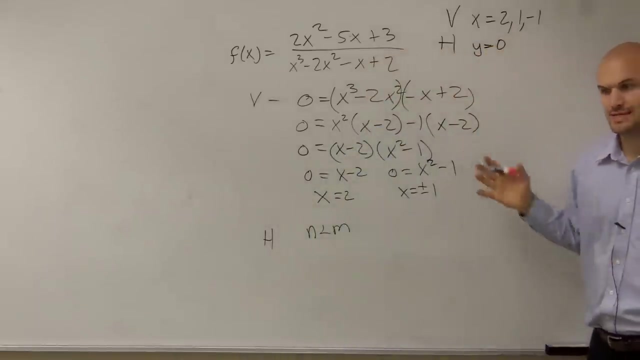 degree first and then in descending order, And what I notice is my degrees, which is 2, and a 3,. since the degree in my numerator is less than the degree in my denominator right, We have a horizontal asymptote at y equals 0.. All right, So that's it, Just by. 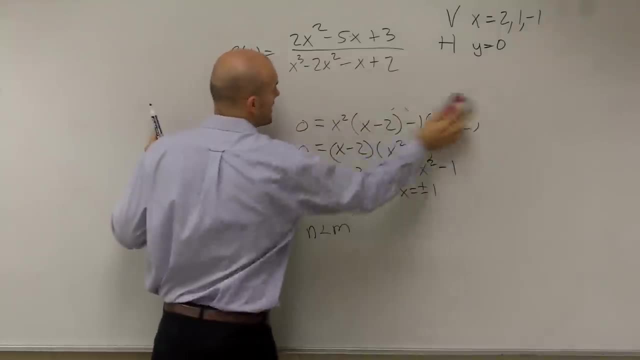 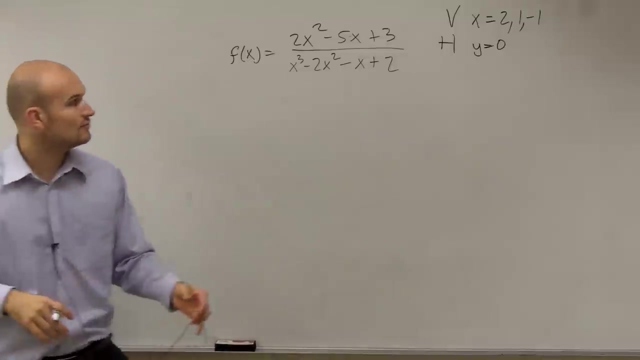 using that test, no mathematics or algebra needs to be used. OK, So you have y equals 0 as your horizontal asymptote, and vertical asymptote is x equals 2,, 1, and negative 1.. Now the next thing I need to do is determine the horizontal asymptote, So I'm going to 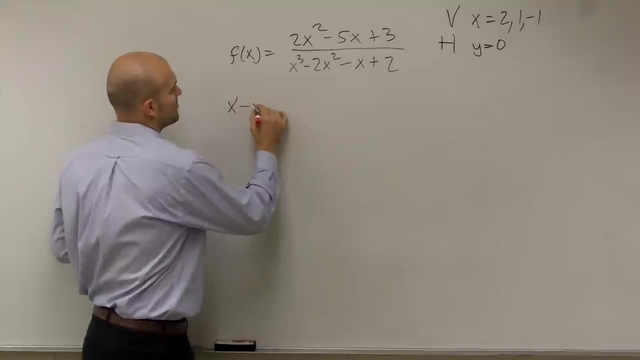 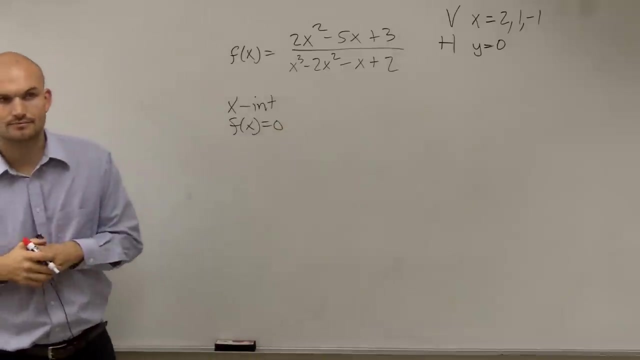 do is it says: define the x-intercept. So remember, in those other problems we worked with, x-intercept is when your f of x equals 0. So what I'm going to do is I'm going to say 0 equals 2x. 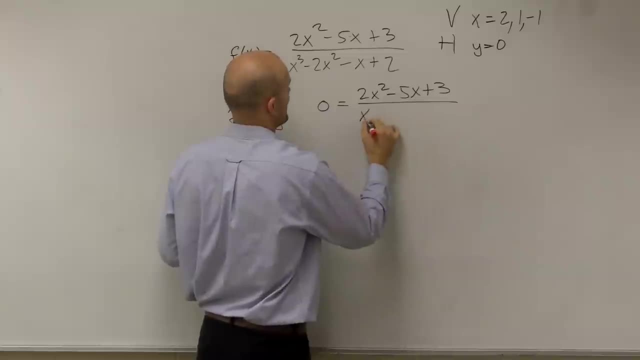 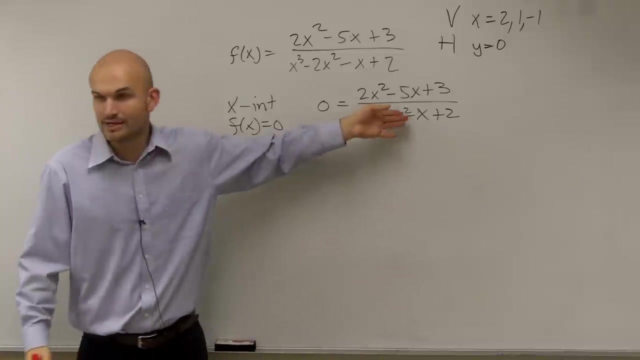 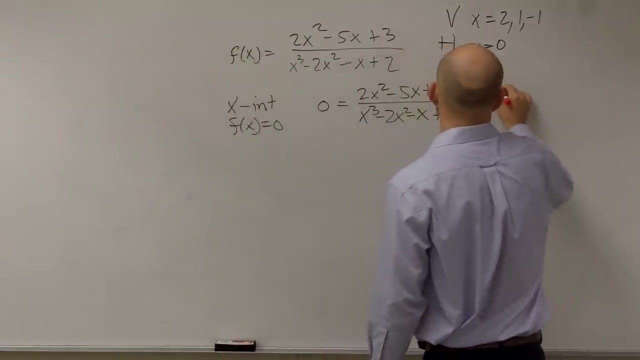 squared minus 5x plus 3, divided by x cubed minus 2x. squared minus x plus 2.. And remember we talked about this: How do we get a fraction off our? you know the bottom of the denominator? You have to multiply it on both sides. So I'm just going to write it really quick: You. 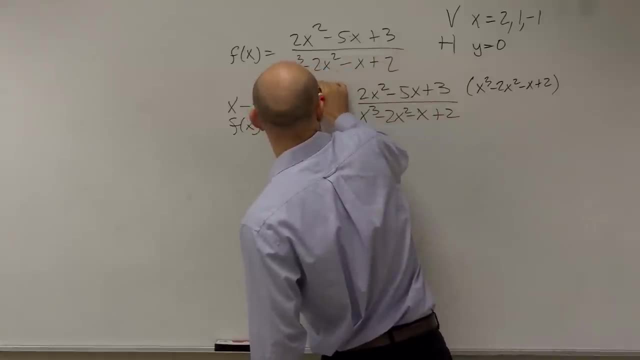 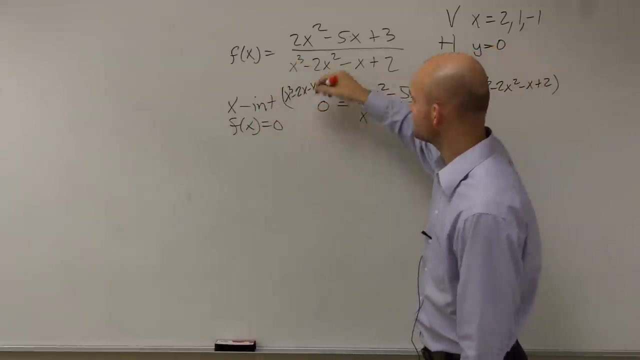 multiply that on both sides, This whole expression multiplied by 0 is just going to become 0. And then obviously, that divided by itself is just going to give you 1.. So you're just left with 2x squared minus 5x plus 3.. Now you've got to say: all right, I'm going to 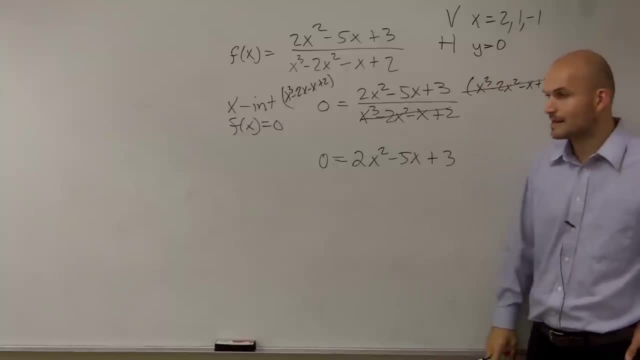 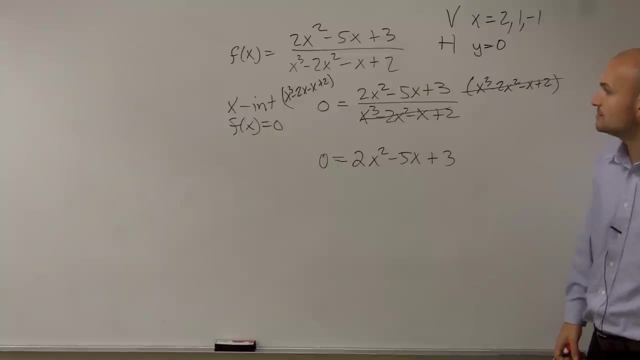 see if I can factor this. So you need to look at this and say: you know what two terms are going to multiply to give me, well, 6?. So I need to look at this and I need to say 2x times x And I need to multiply to give me 3.. Or look up there and give me 3.. So it 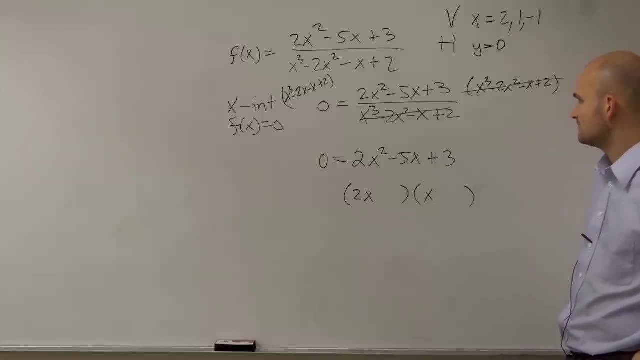 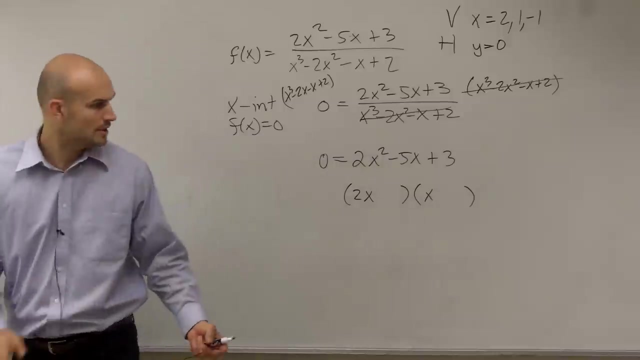 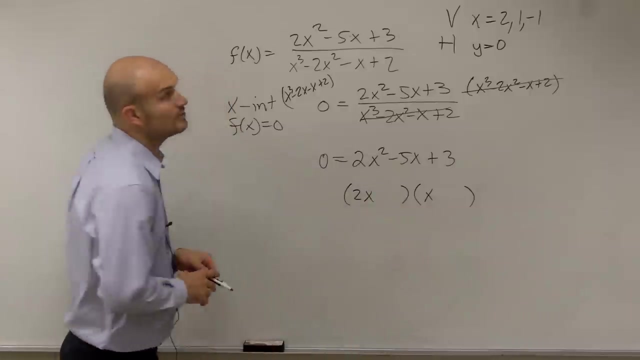 So it would be. I'm not seeing that's factible. So then what? I'll look. I'm sorry, But the only problem is negative. well, negative 3 and negative 1.. Actually, no wait, could you do negative 1 and negative? let's do this: negative 1 and negative 3.. 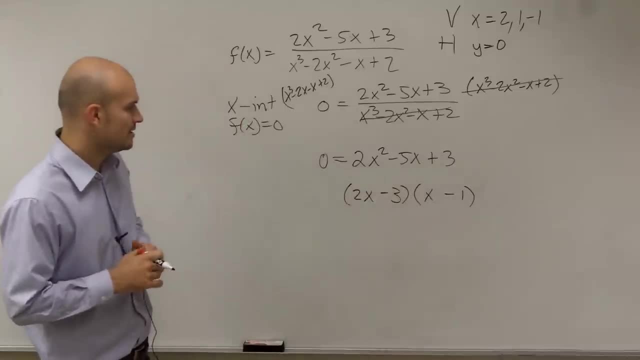 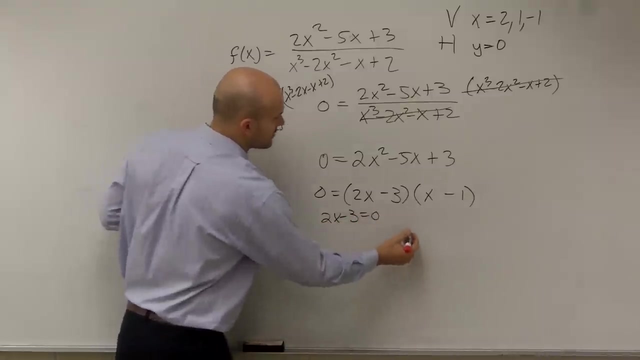 Yeah, well, I was thinking about switching them the other way. That's what I was looking at, But that will work right? Yeah, that works. There you go. Equals 0.. So, therefore, your x-intercepts are going to be now. so now you say: 2x minus 3 equals 0, and x minus 1 equals 0.. 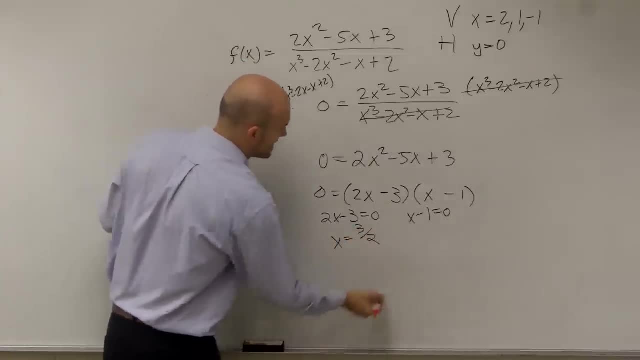 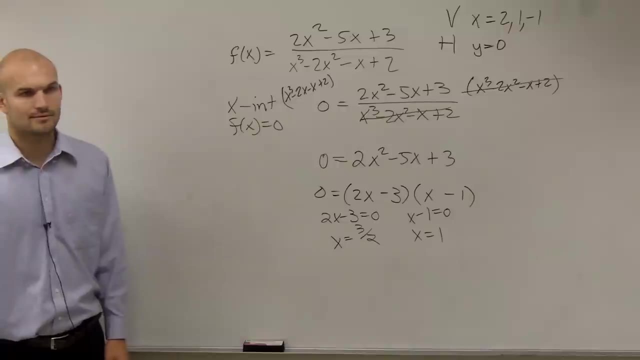 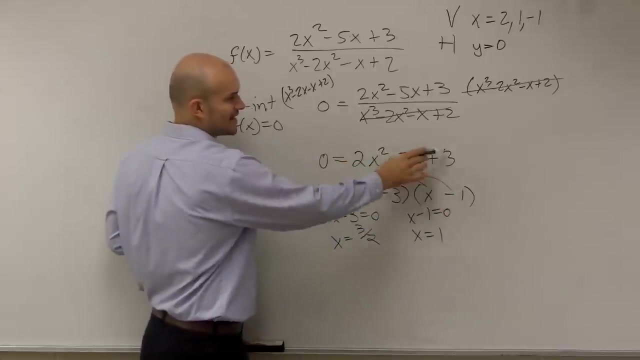 So now you could say: x equals 3 halves and x equals 1.. What's that? Yeah, Remember, you're multiplying these right 2x times x is 2x squared right, Negative 3 times negative. 1 is positive 3.. 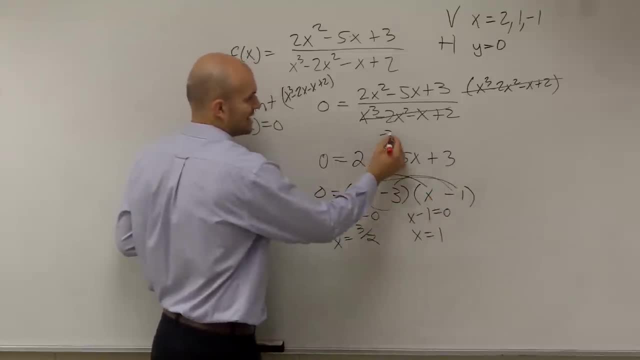 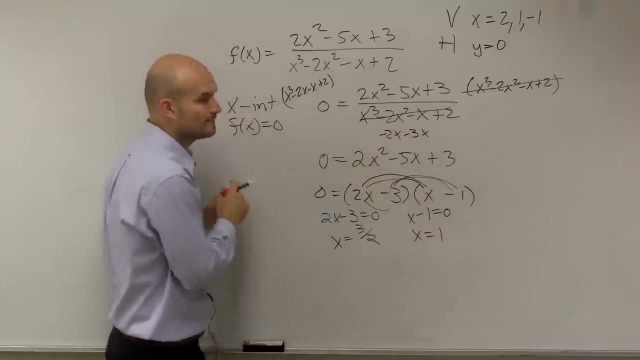 2x times negative. 1 is a negative. 2x Negative. 3 times x is a negative. 3x Negative. 2x minus 3x is negative: 5x. Okay, So are we cool with the x-intercepts? 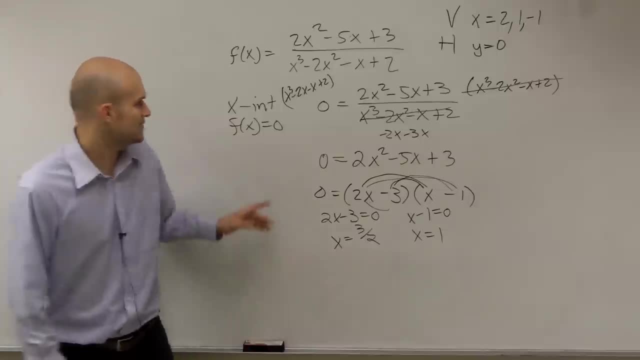 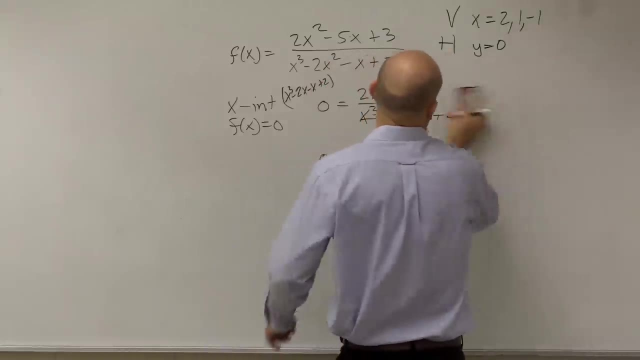 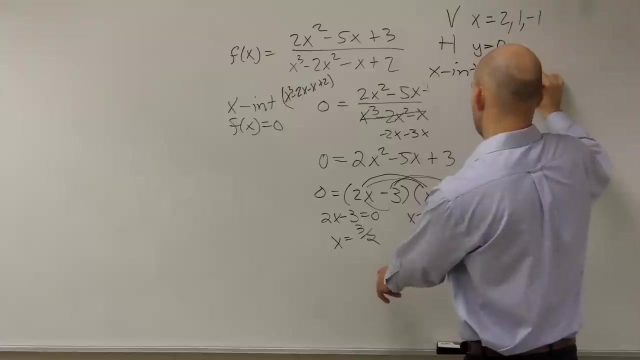 Because now we need to do the y-intercepts. Actually, we can do y-intercepts right here. I want to do them below. So we could say: the x-intercepts are: when x equals 3 halves and when x equals 1.. 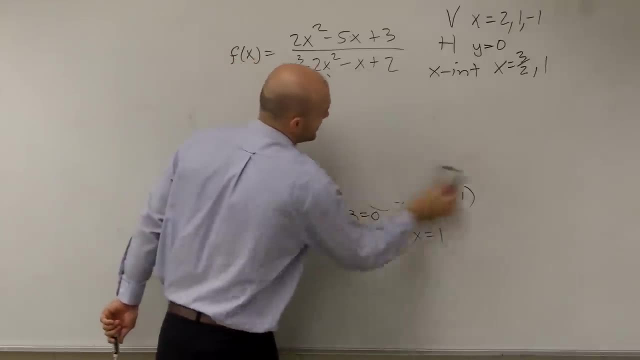 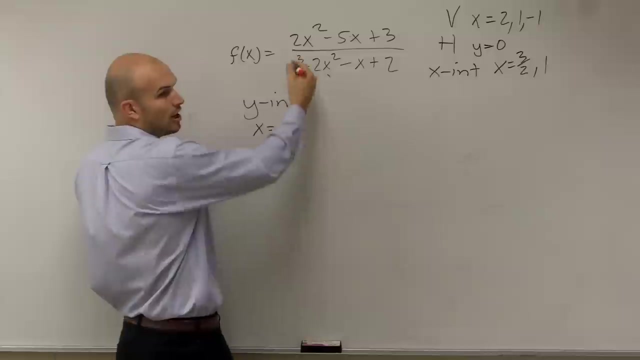 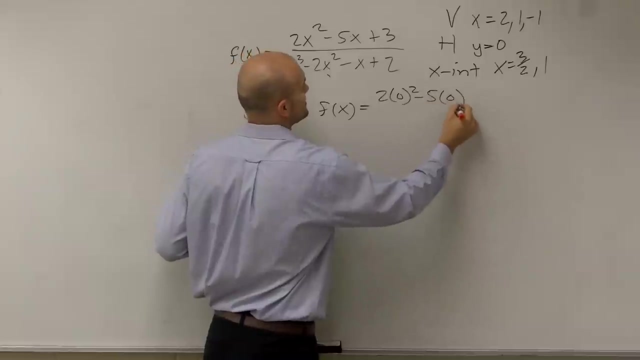 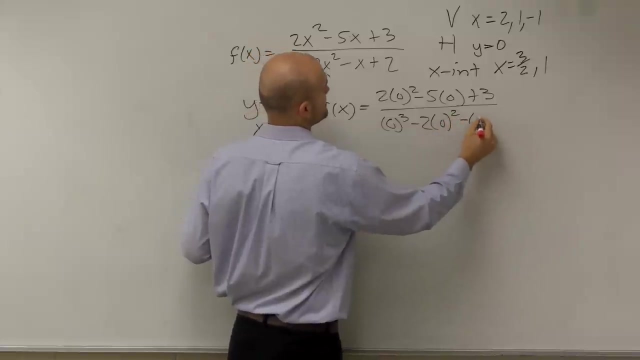 So the last thing we need to do is now determine the y-intercepts. So to determine the y-intercepts, that's when x equals 0. So all we do now is plug in 0 and for x. So you do 2 times 0 squared minus 5 times 0 plus 3, all over 0 cubed minus 2 times 0 squared minus 0 plus 2.. 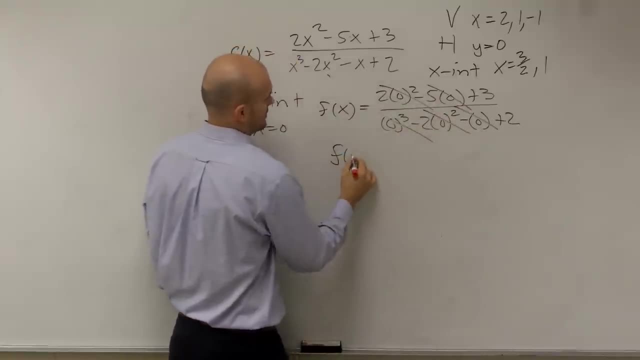 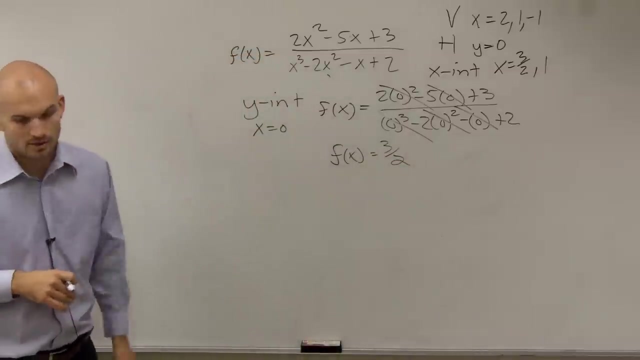 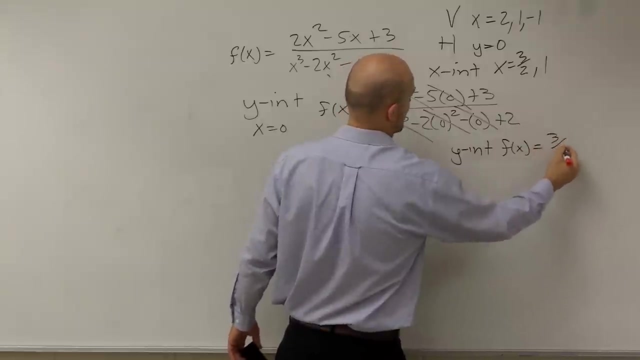 0, 0, 0, 0, 0.. Alpha of x equals 3 halves. So to finish off the rest of this problem, you can say your y-intercept, Which I didn't leave room for- Your y-intercept is when alpha of x equals 3 halves. 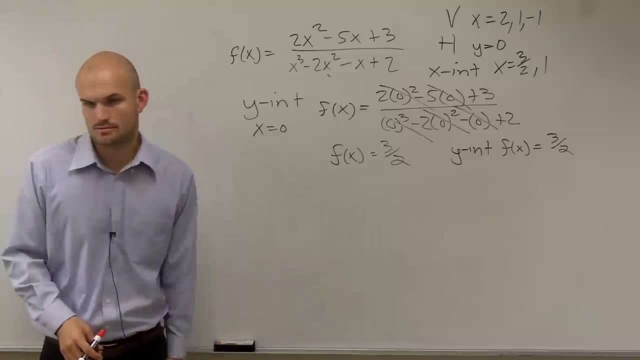 Any questions on this? No Good, Maybe Okay.